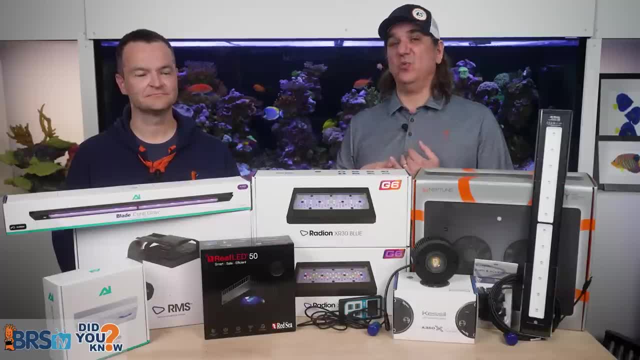 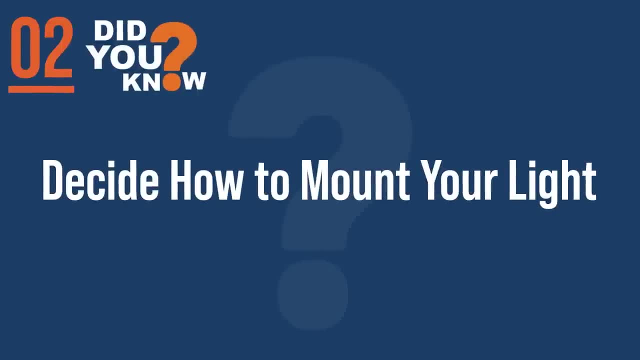 We're going to get the paw right with the schedule And then we're going to have the confidence that we did it right. so we can just leave it alone. Let's do it. Number two: decide how you're going to mount your light. 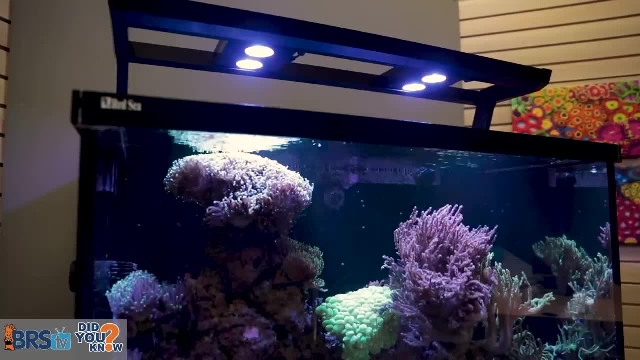 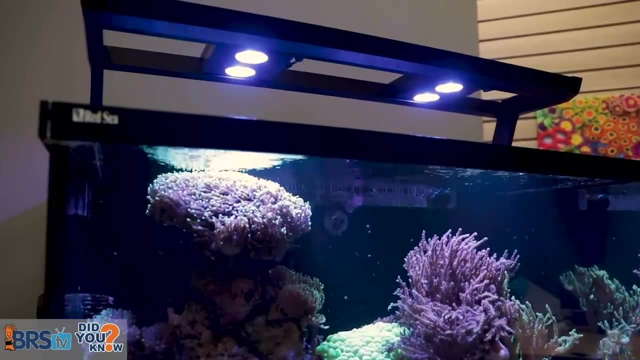 And this can be confusing for beginners. so let's make it really easy. If your light has mounting arms or legs, just use them. They're easy and they should already be near the ideal height. Okay, it's not always true that they're the right ideal height. 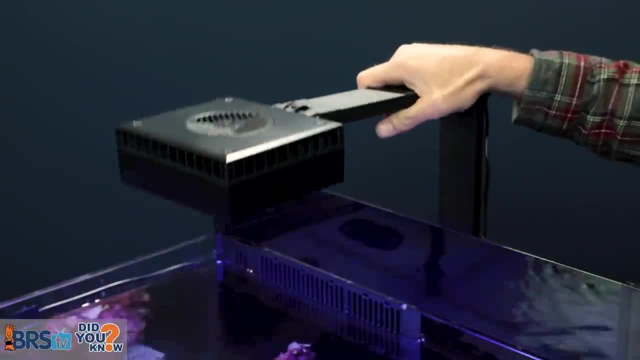 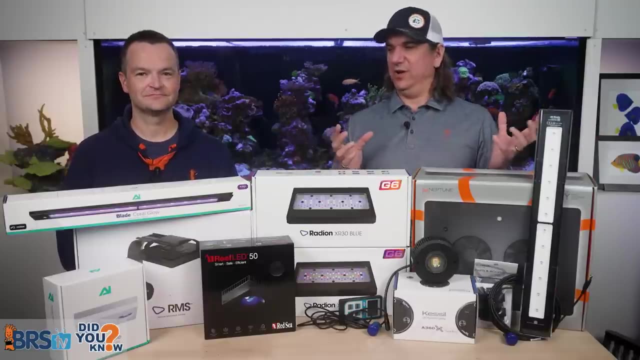 But if you're buying it from anybody reputable, the mounting height of the arms is actually designed to the light, so it should be So, I think, a vast, vast majority of people. if you're trying to figure out how to mount it- and it comes with a mounting kit- 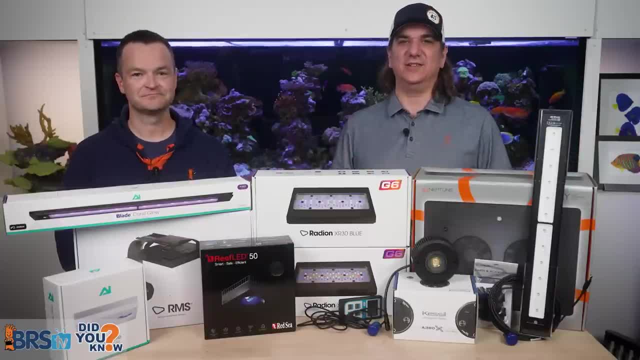 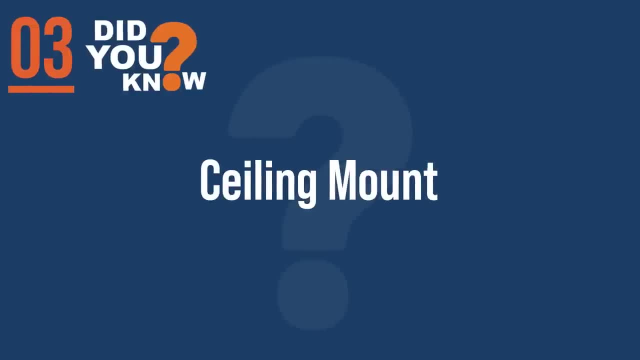 That's designed either in the box or is optional. you'll probably use that. Number three mounting to the ceiling is one of the rarest ways to mount it, but it's actually one of the best as well. I know it can be a little intimidating. 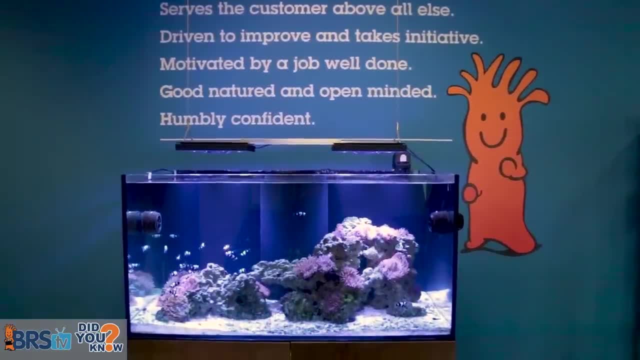 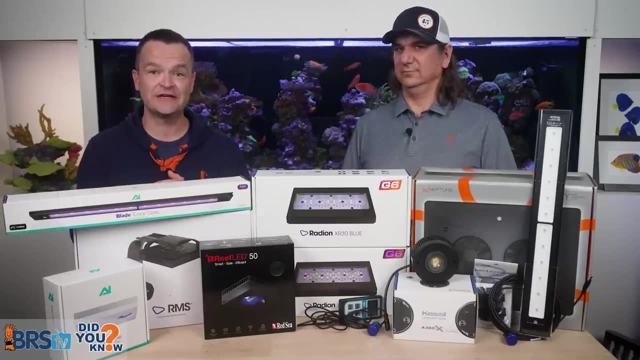 So here's a couple tips for you. Centering is the most difficult part, because you get it up there and then it's just barely off and it's going to bug you forever. So one really simple trick here is just use a string and tie a washer to it. you know, hold it up at the ceiling and you'll see exactly where. 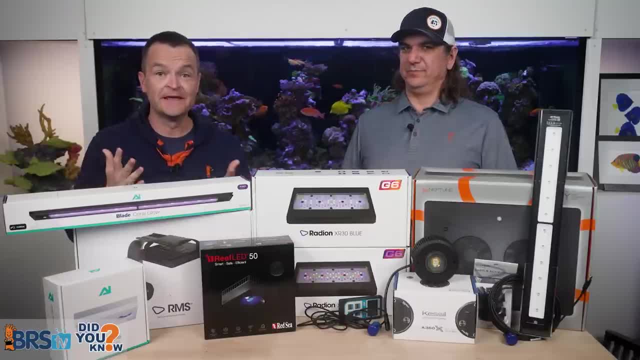 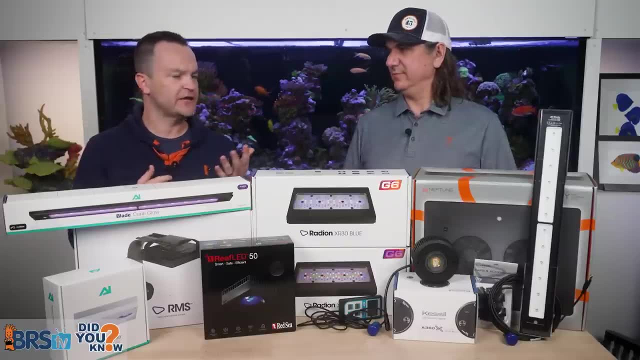 that washer sits. Then you can just take a pencil and mark the center done to actually mount that to the ceiling. There are a couple of ways to do it. One: if you just have some drywall up there and there's no stud nearby, use some toggle bolts- really easy way to do it. 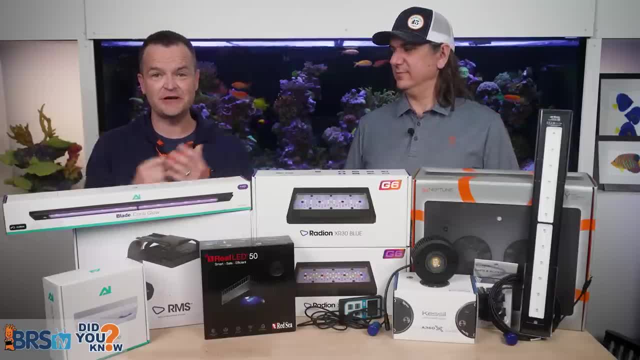 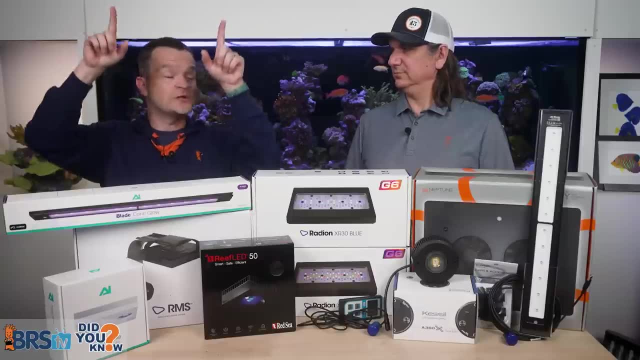 But if you want to be extra sure- and it's in those studs, but there's no stud right there- all you need to do is just take a piece of wood- It can be a two by four, whatever you want, you know- find the studs, drill into the studs and then paint it to match your ceilings and just hang it from there. 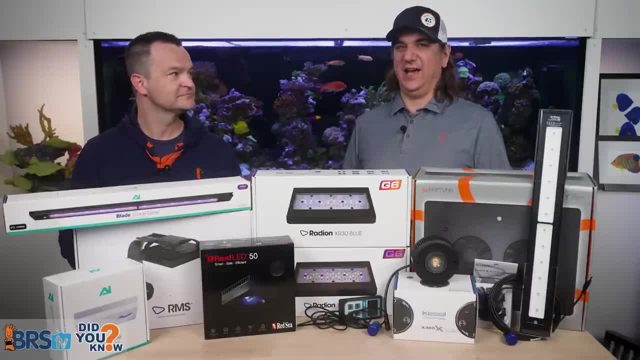 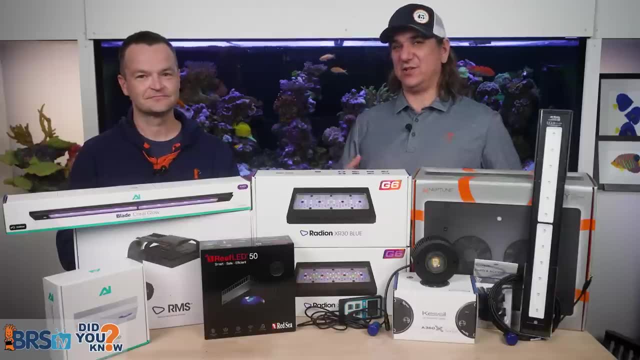 So I will tell you, I did this for myself My first time on my first tank. I got sick of the little legs that were breaking off of my little Coralife fixture and ultimately they replaced it with a T5 fixture that really only had the option to hang it from the ceiling. 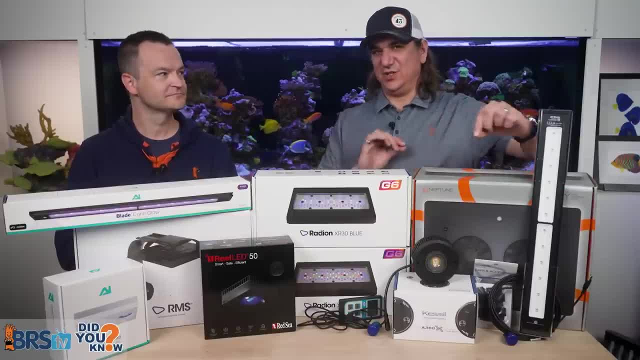 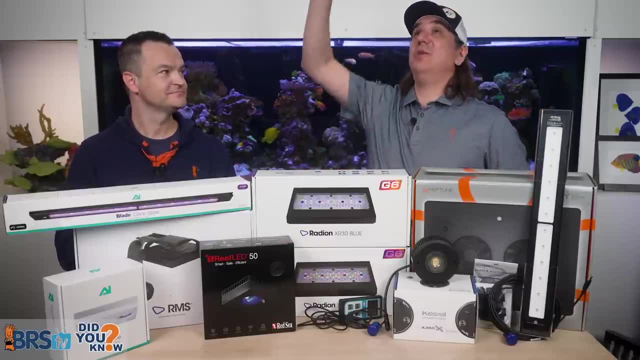 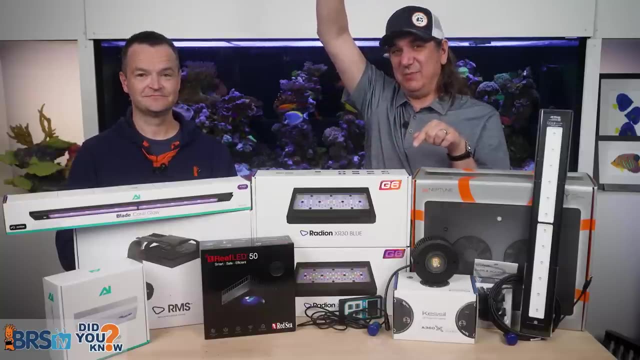 Intimidating at first, until somebody in the local club told me to do this. Just take a piece of tape and then tape where you have the holes on your tank intersection, and then go up to the ceiling and hang that piece of string until the washer at the end of it is centered right over the pieces of tape. 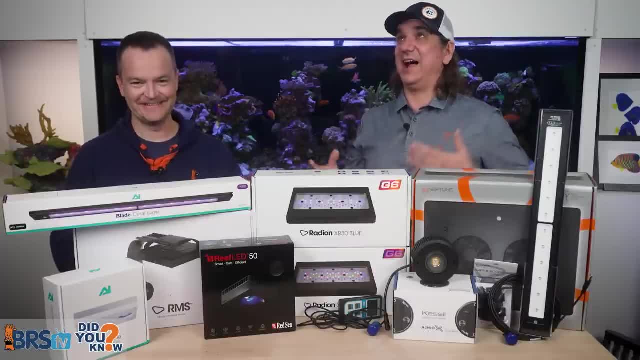 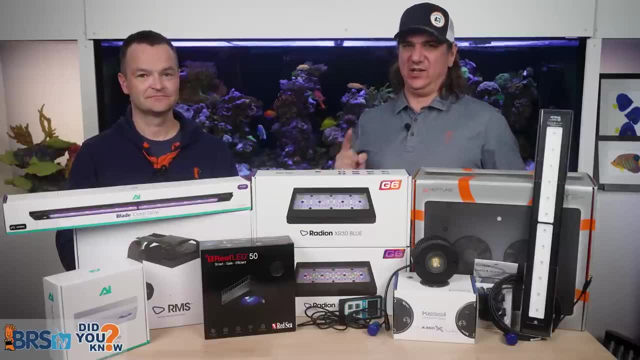 Yeah, And now it's perfect. I was terrified prior to that, Like how am I ever going to measure this right, That it doesn't end up looking wonky, and set up my OCD after I did. It was really easy. I use a little toggle, bolts, drill hole and a snap open. 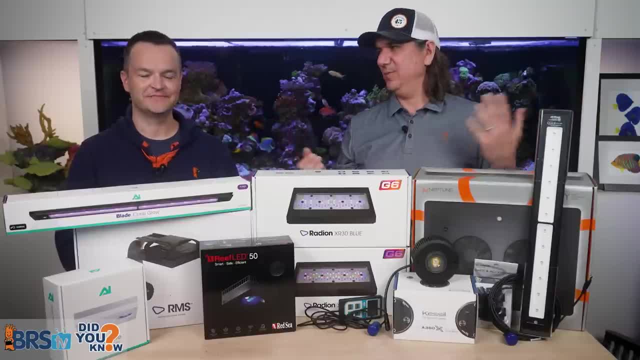 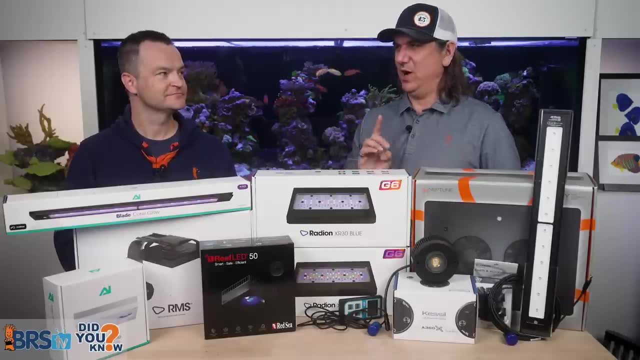 I mean, they hold a lot of weight. So the typical light that we're using is an issue You could. you could do the plywood method if you wanted to, and really secure it. But here's the thing that's really cool: Why, Like, even though you know some, obviously some of you don't want to go through this effort. 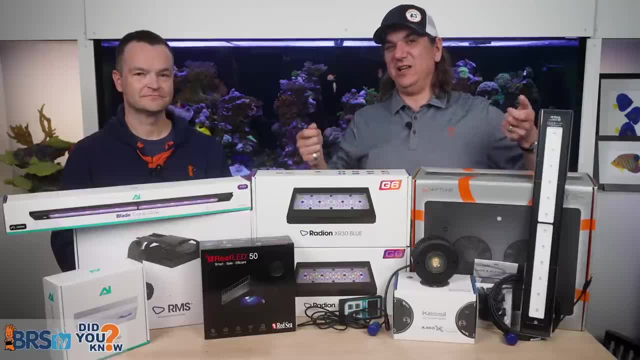 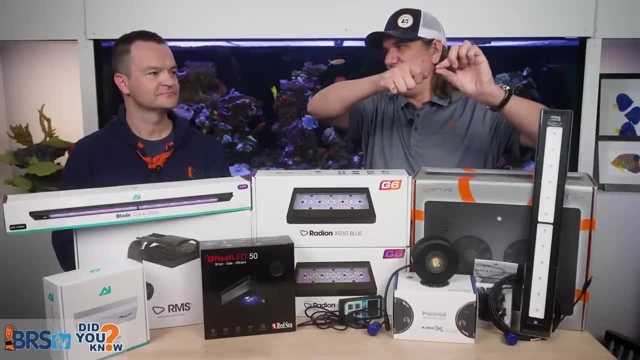 What's really really cool About it is now when I need to get in there. I don't have to like take these lights off or do anything, especially if I had a big fixture. I just pulled a little line on the cable and it goes and zips right out of the way I can get in there. 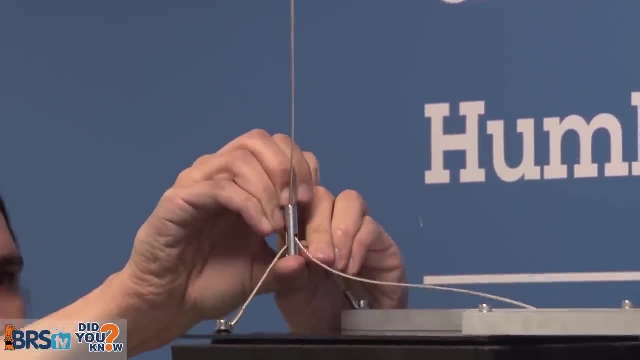 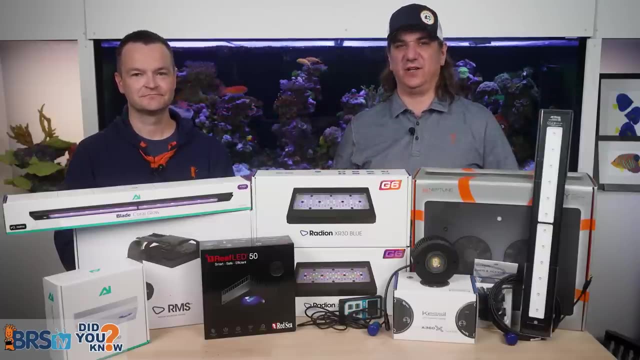 And then when I'm done, I push the little button and it slides right back down to where I wanted it. It's one of the best ways long term, because it gives you really easy access to the tank, especially on big fixtures. Number four: there's actually wall and tank brackets out there. 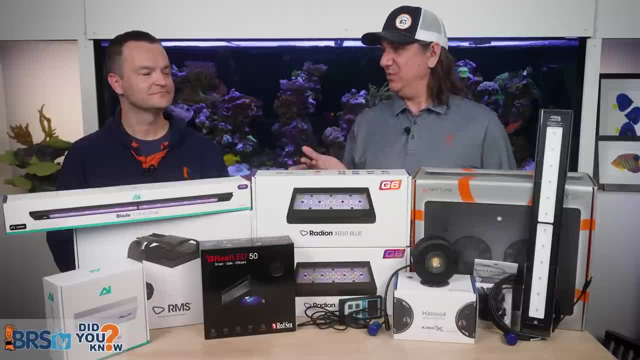 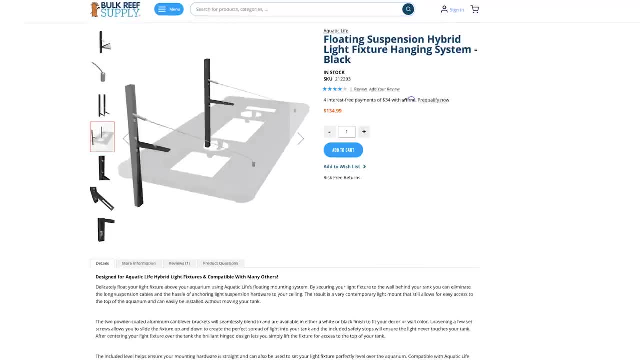 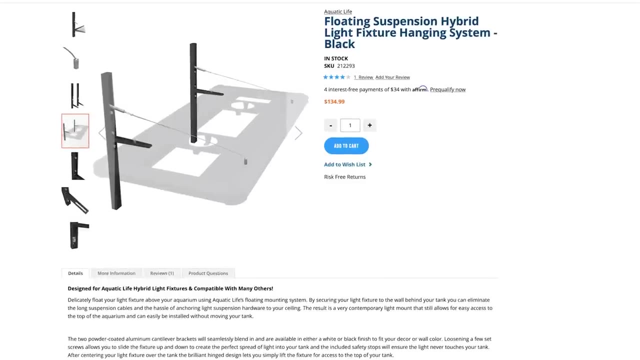 You can choose to mount to, many of which may be tied to a brand but can be used for other brands if you want as well, starting with the aquatic life floating suspension system. So what that does is you bolt a little bar to your wall and then it has a cable that comes out and, like you know, hangs it like a suspension bridge. 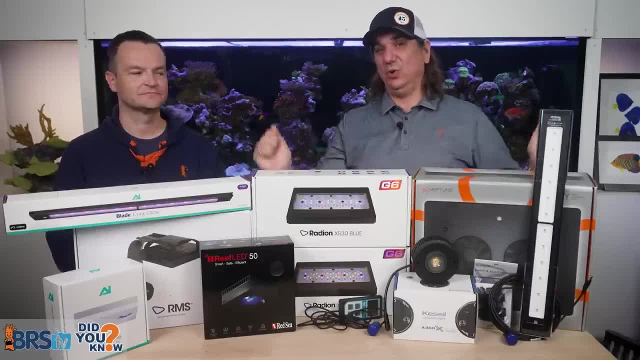 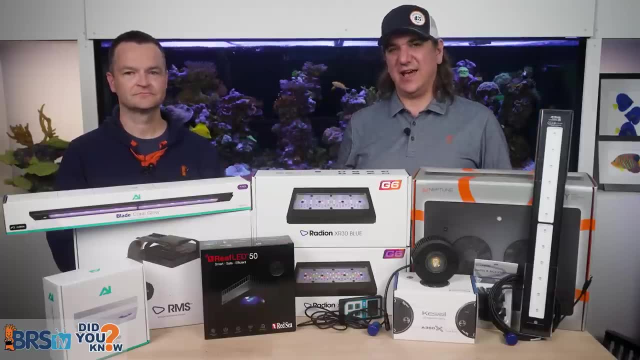 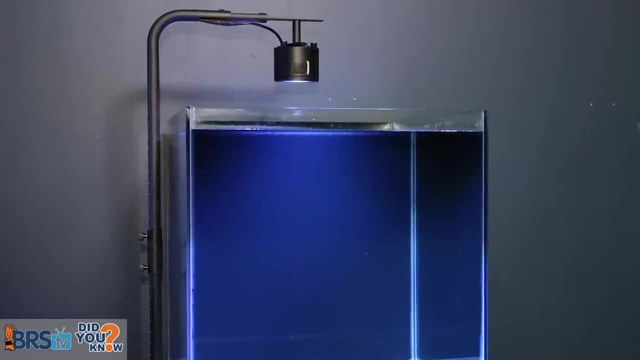 Yeah, And now I have the ability to have that cool suspension that I can lift in it and take it on and off the tank or raise it, but it's attached to the wall. Another option like that Is a Kessil's option, where you can like bolt it right into the stand and then the arms come out and over. 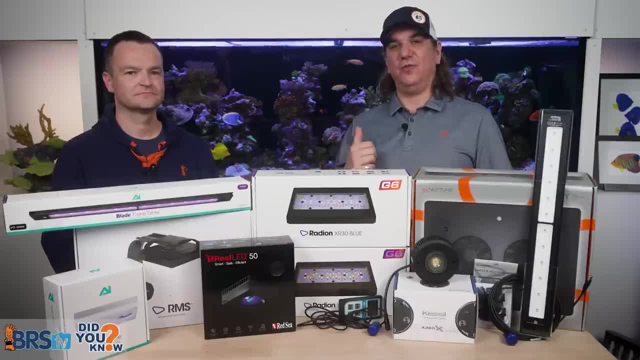 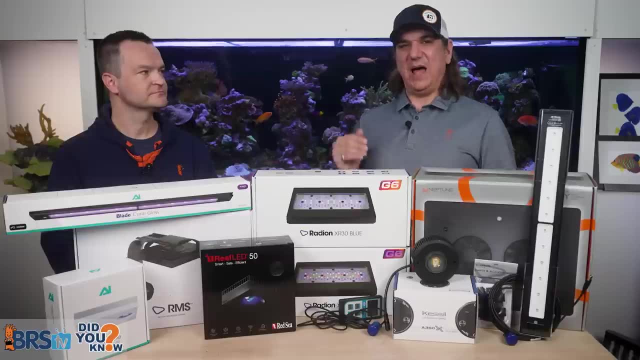 So really strong options. There's also options that go into the wall for that. Even AI has the HMS system for something similar to that as well, So you can mount it to the stand, have arms that come out, you can have multiple to the wall. 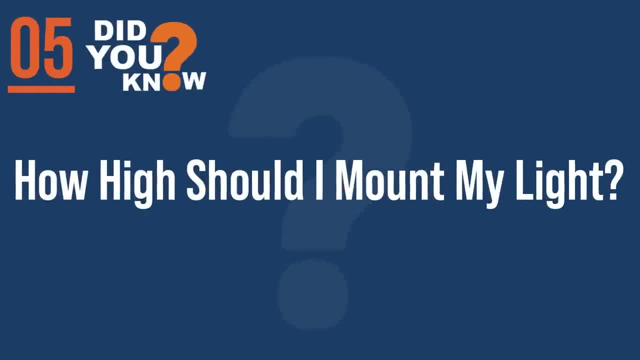 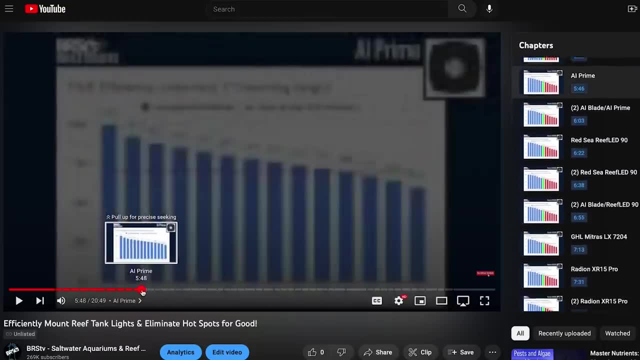 It's all kinds of cool options for the brackets as well. Number five: how high should I mount this light? It's a really great question. Well, you can Watch our positioning of light video. It's long. It has like 50 lights in there, but they're each timestamps. You can find the exact light that you have. Mounting height really matters when you're talking about a small fixture- I mean, there's not a big window there where it's working at its best. It matters less definitely when you have a larger fixture. 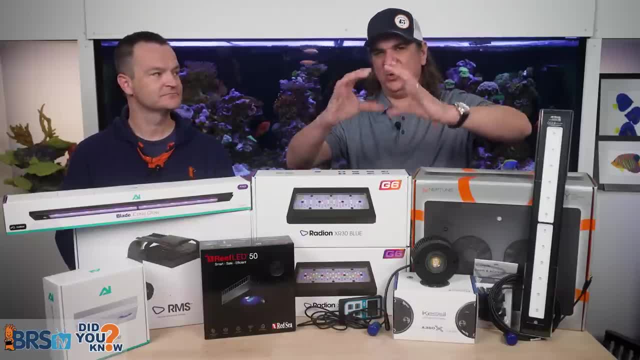 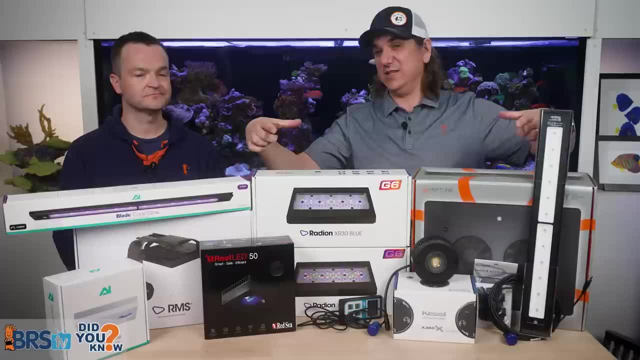 Yeah, So mounting height matters. for this reason, If I have a little small module, it's basically got like a cone of light coming out of it, So I mounted it fairly high. You know it's got a cone that covers the whole space. 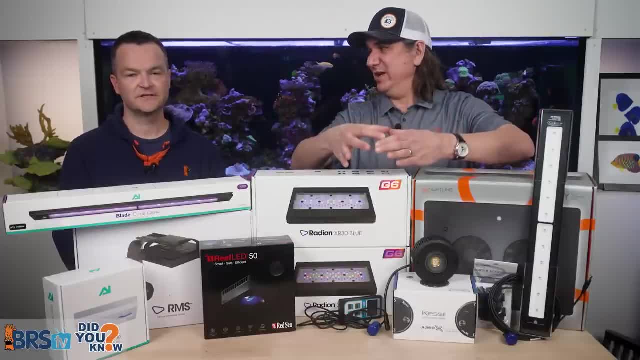 But if I mounted it too close, well, that cone is not creating like a laser beam, you know. So instead of like having a whole bunch of points that are 100 par, I got a whole bunch of points right in the center that are 1000 par. 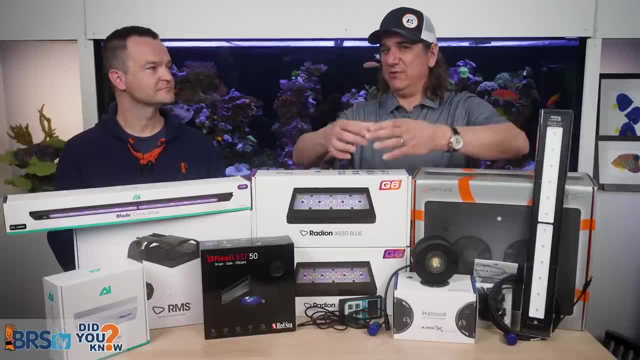 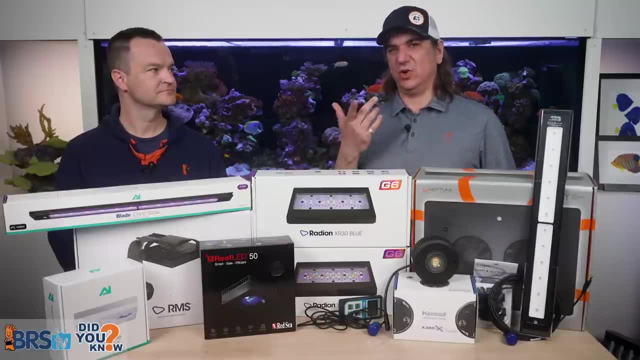 And I'm just going to burn and kill everything, And so that's why we have a smaller one. It's really, really important to get that mounting height right, And what we're doing in the positioning of light video- so go watch that when you're doing this- is you can find either your light or something like it, because there's, you know, 50 of them and it's covering. 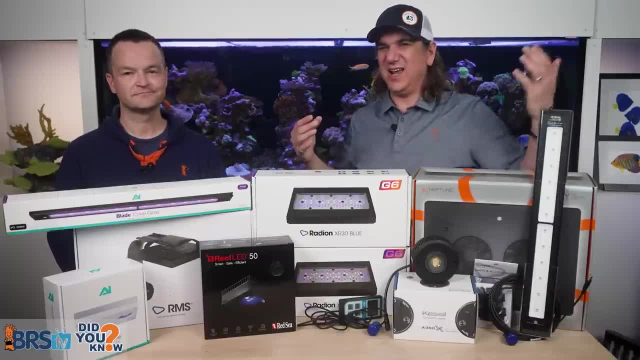 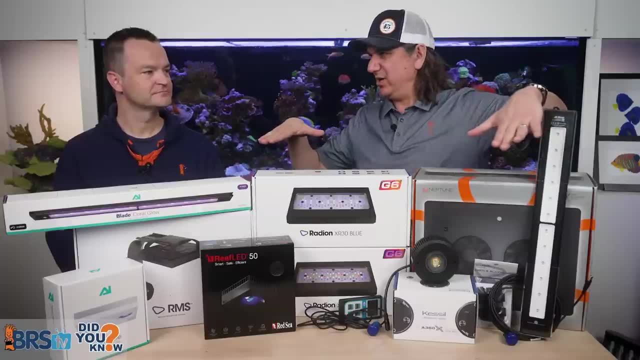 Over a two foot area, which is a pretty common space. You can kind of take a guesstimate if it changes out that, But what we're really looking for is a balance of let's get even spread across the top without spilling too much light into the room. 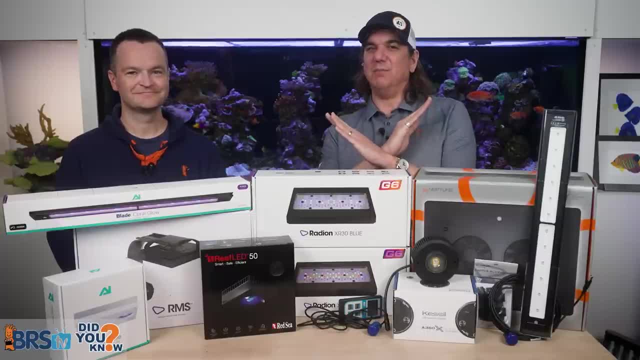 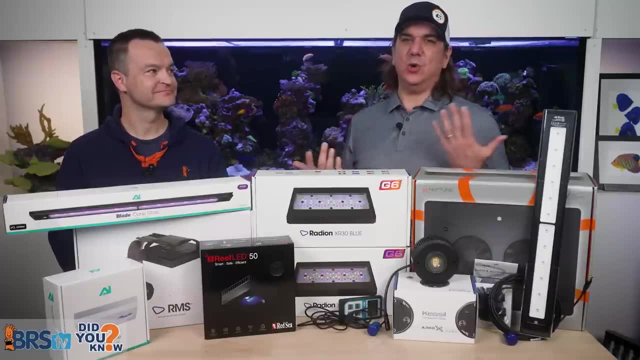 And the answer is the intersection where we don't do neither of those Absolutely perfect man, But we do both of them really, really well. That seems to be the intersection where we're going for it, So go watch that if you don't have that available to you. 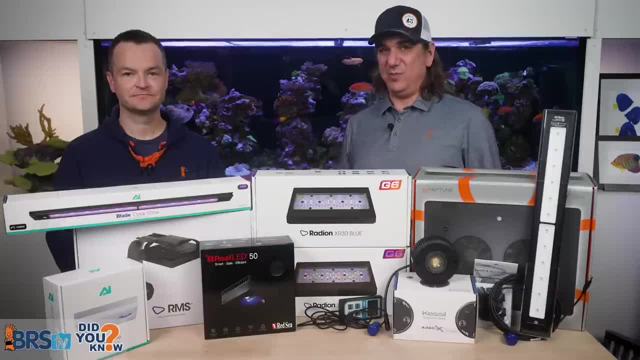 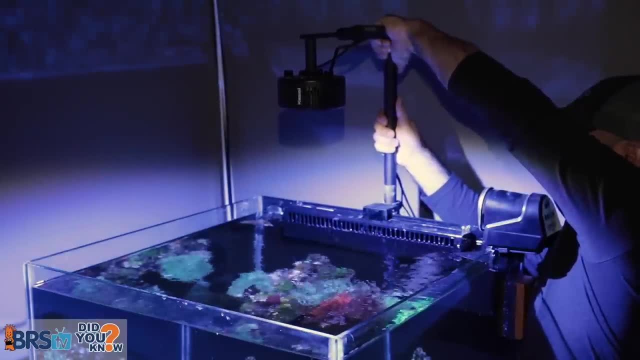 Obviously a par meter is right, And if you don't have a Par meter and this doesn't exist for you, Literally just lifting the light up and looking at how much light goes into the room and how it's kind of spread it out in the tank. And if you don't even want to do that, most of the lights out there I will say fit pretty well inside of like a, you know, 78 inch window. You know a couple of them a little lower, a couple of little higher, but seven to eight inches is pretty safe, unless you see those little lenses on there. 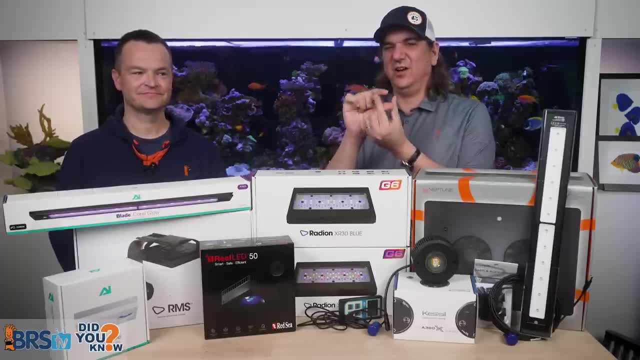 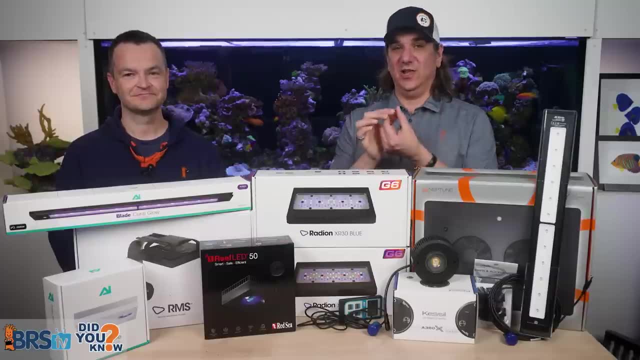 If you see those little commodity like White lenses on there most of the time and you're looking at like 20 inches, This thing is a focus lens designed to shoot way, way, way down. So if you see those little lenses mounted high- everything else in any case- 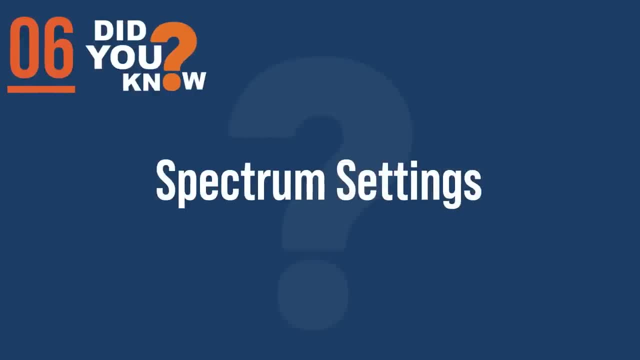 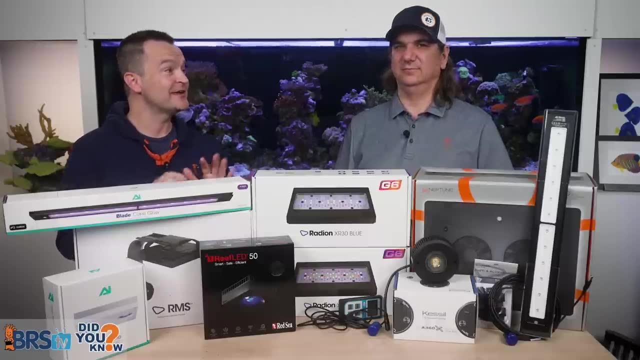 So you can see the importance of actually getting this right. Number six: what about spectrum settings, All those switches, all those individual lights? How can we get it right? Well, using a preset is going to be way better than just individually flipping switches and changing each individual light. 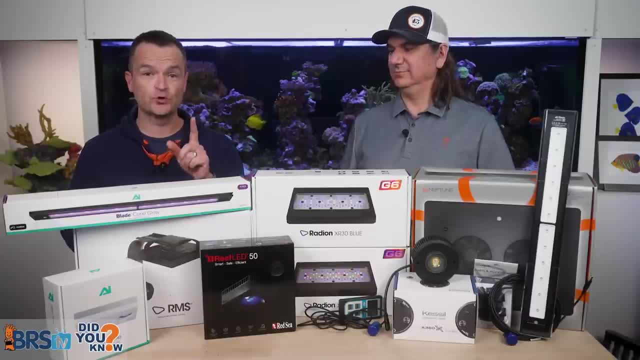 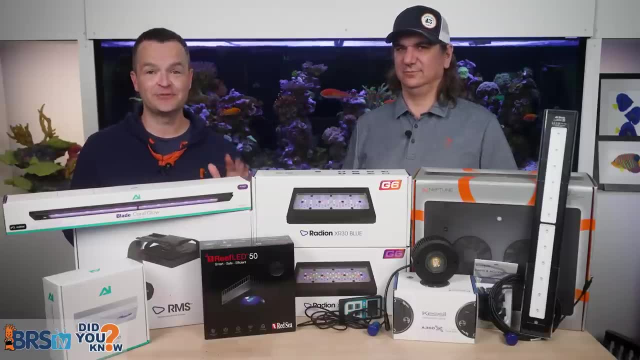 Remember a few key facts here. Blue is for your coral growth, White gives a lot of beautiful colors, Green will actually make things look brighter, and red Well, that's for the trailblazers out there. You can have all of these change throughout the day, but you're more likely to mess things up. 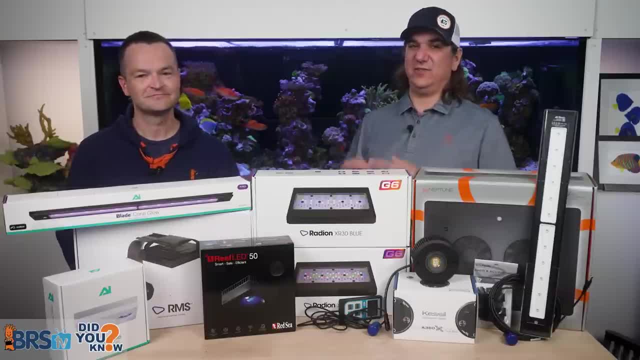 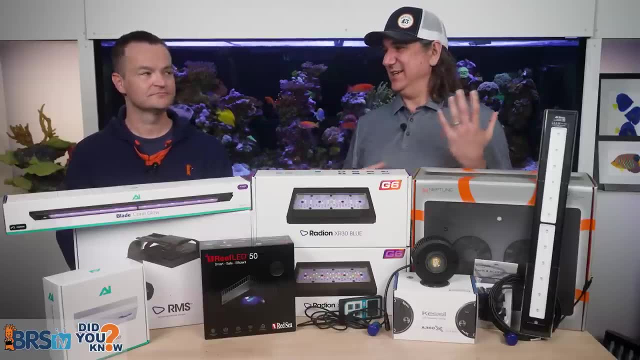 So keep it the same. Yeah, that's a big question is like: should I have a different setting for the morning and the evening? And the answer is: you can, but really the coral has to adapt to those changes, So the less the coral. 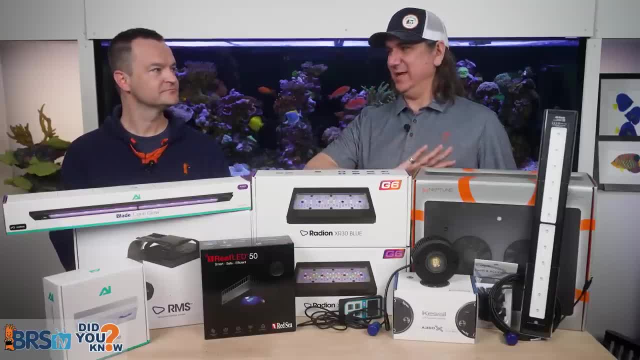 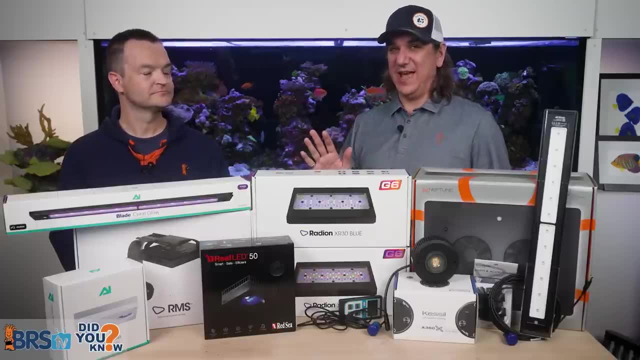 Less to adapt, the better. So if you actually did have largely the same spectrum throughout the day, you'll probably have more success than not. It's not that you can't have different ones, It's that it's just a little bit of the wild west now, because everybody's just kind of like guessing. 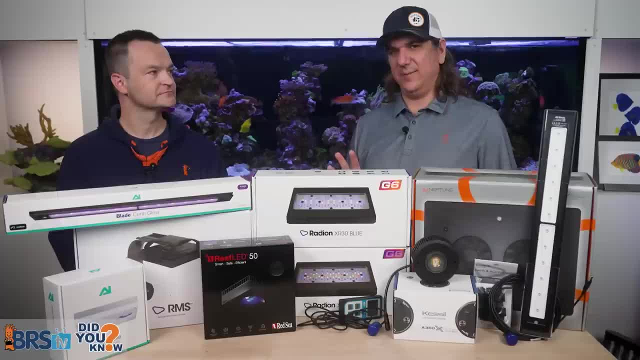 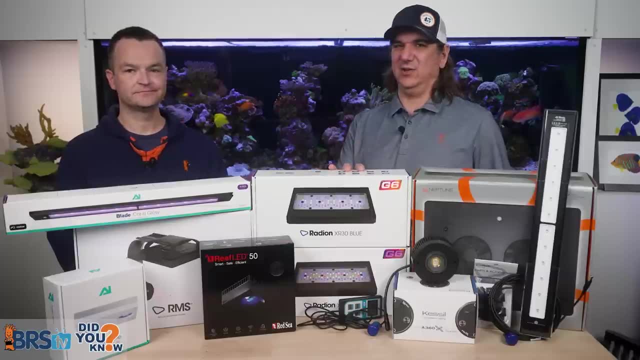 And I guess what I would say is those presets that come in there. or for people who just want to plug it in the wall and have it work, pick the preset. like with the Radion, There's the AB plus. You know, this is like proven out inside of farms and stuff. 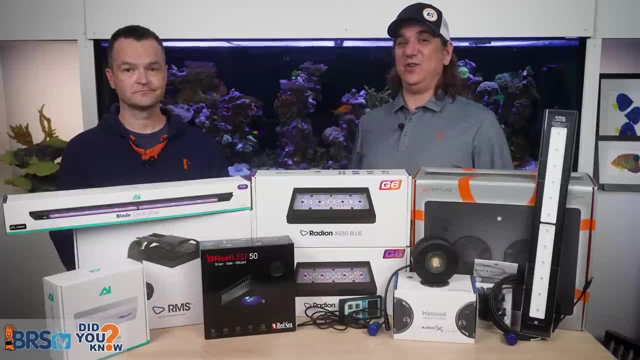 Uh and Just use that Uh, and then if you are the type of person where you know what I don't want, to actually just plug in the wall and have it work, then I'm going to actually willing to risk the fact that it might not work as well to achieve, like a very specific desire. 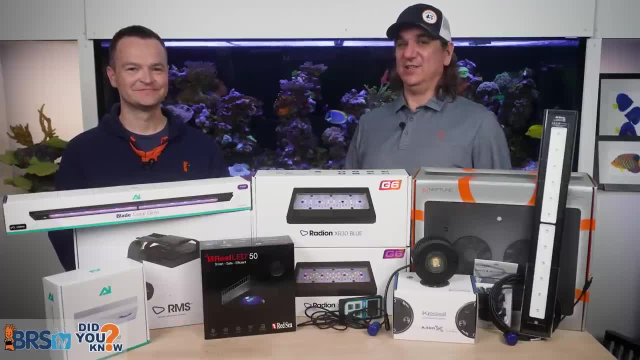 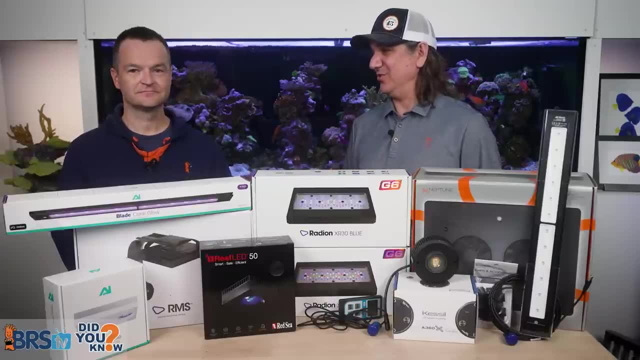 And you better know what that desire is, because this is not for your eyes. This is to support biology, for an animal right That survive needs this light in these ratios to survive, or it will have to adapt to the new ones that you create. 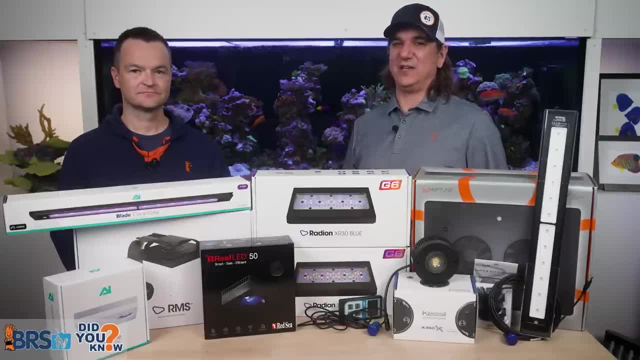 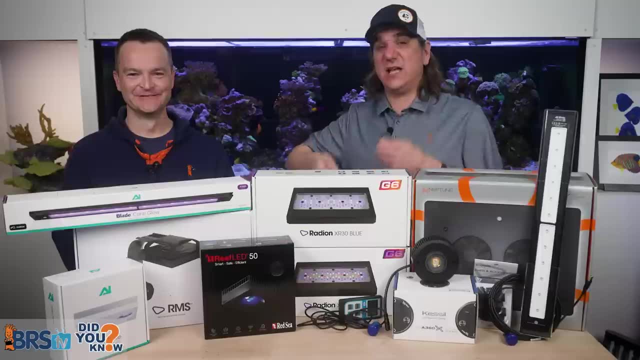 So the spectrum settings: Use the preset in a vast vast majority of cases and then just leave it alone, And that will produce the best results. One more time: leave it alone. Every time that you switch it expect things to get worse, not better. 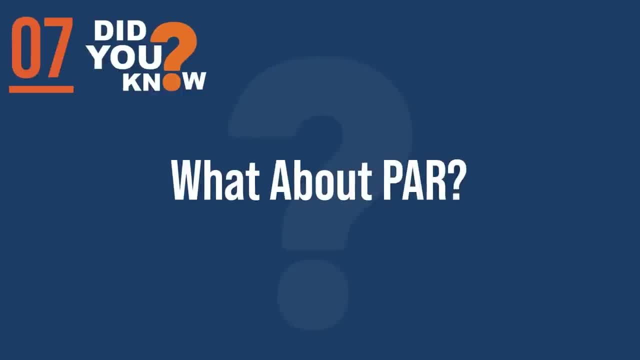 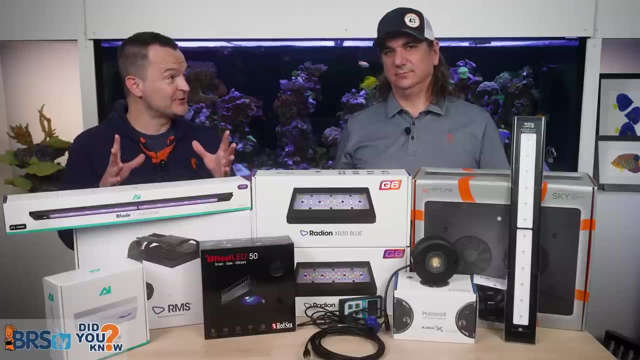 Number seven: What about par use, a par meter? There's actually one that's right around $200 and it's a great option for anybody with a laptop or if your computer is actually relatively close, because the cord on that thing's pretty long. It's the first one I used and it works absolutely fantastic. 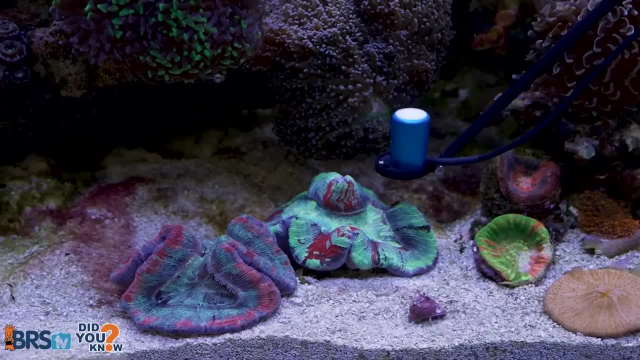 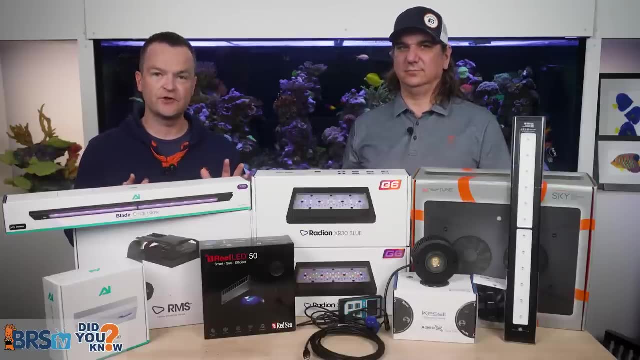 Otherwise, you can just buy one from us and then you can use it for up to 60 days, I believe, and then you can return it And remember the baseline you're going for here. if you have an LPS tank, we usually shoot for around 50 to 150 par, and then for SPS is 200 to 350 par, and more is definitely not better here. 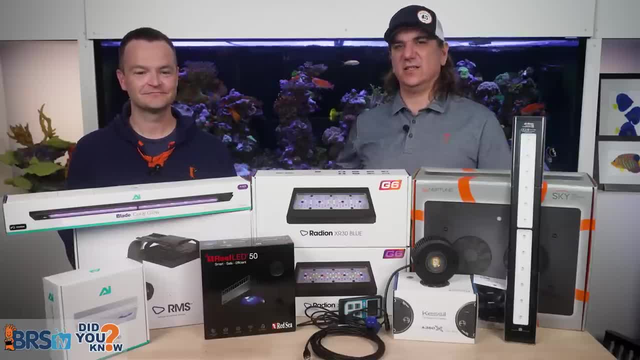 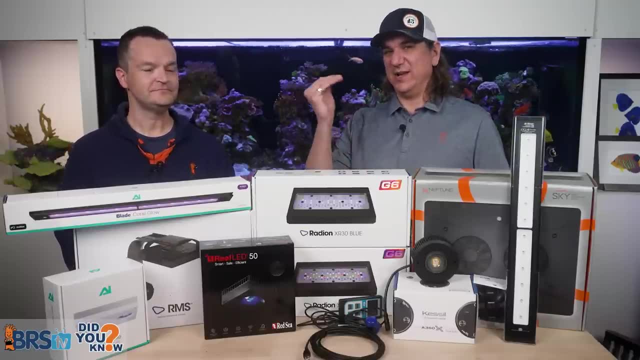 The important part here is the eye can't see this. This isn't something you're going to tune to brightness, because your eye perceives green as brightness And it's like registered brightness. So, like I, like 10 times as much as blue. 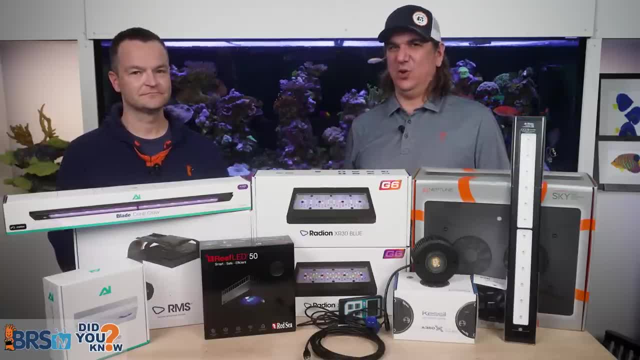 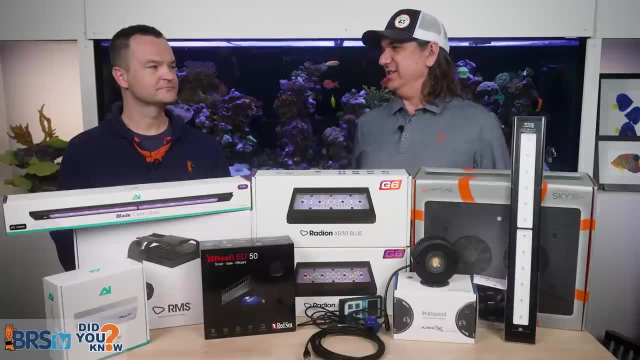 So if we turn off all of the like white lights and only the blues on, it's going to look super dim, but it's probably really high par. anyway, You really can't see this with the eye. We've done- actually did an expert investigates on this? 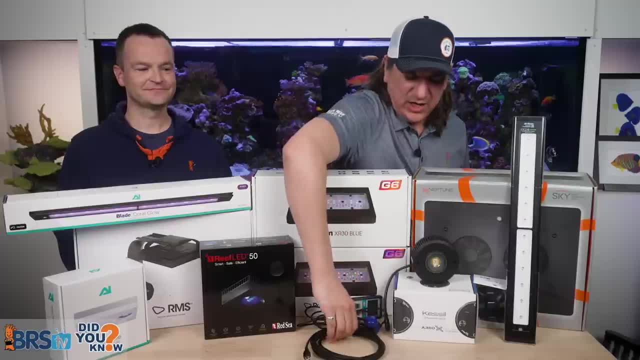 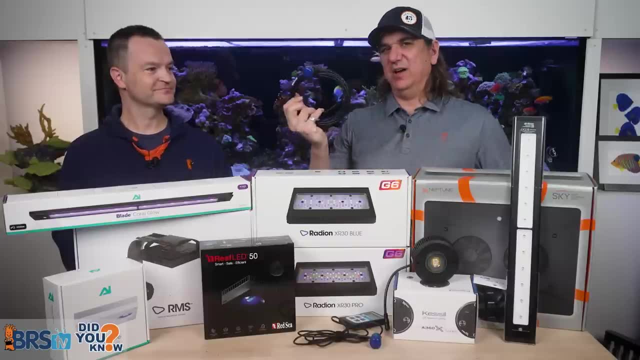 Go watch it. It's pretty compelling. But in any case you know again. you said that this one right here plugs in your laptop. I would prefer to have the laptop near me so I can see it, But 200 bucks, you now have a par meter. 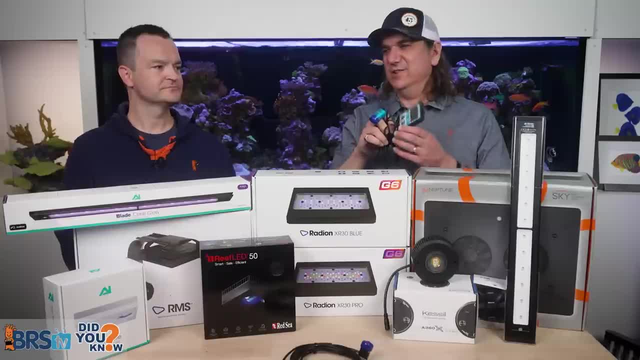 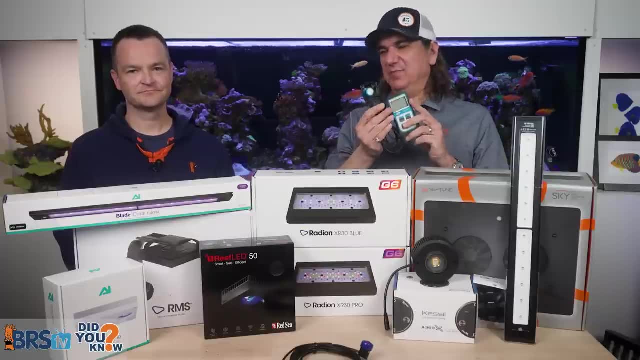 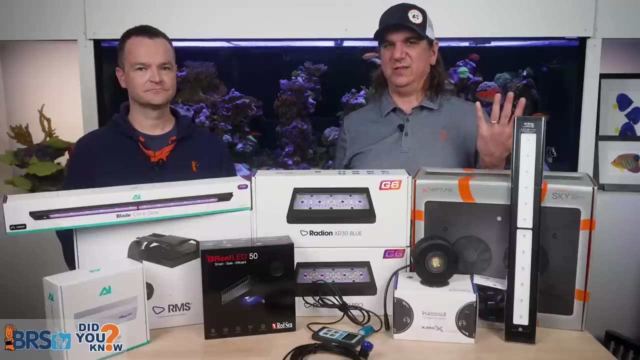 There are, However, sometimes where a standalone unit is just better. I got the little wand for this, I can read it in real time, or whatever. And better yet, these options, right here, these options. We do this as a service for all you guys, because you're going to pick up these lights. 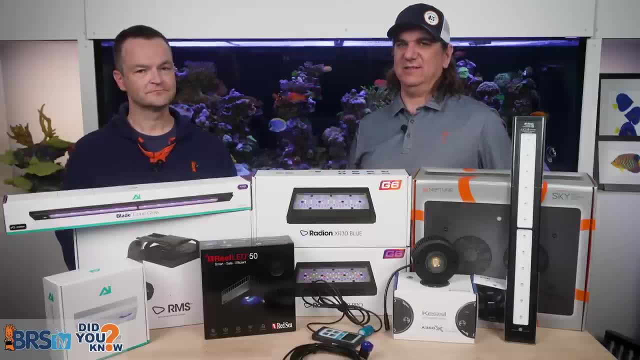 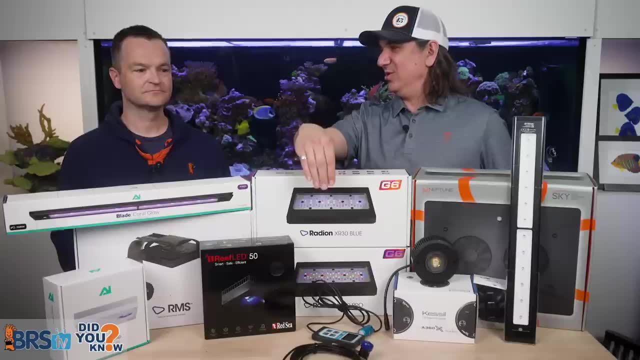 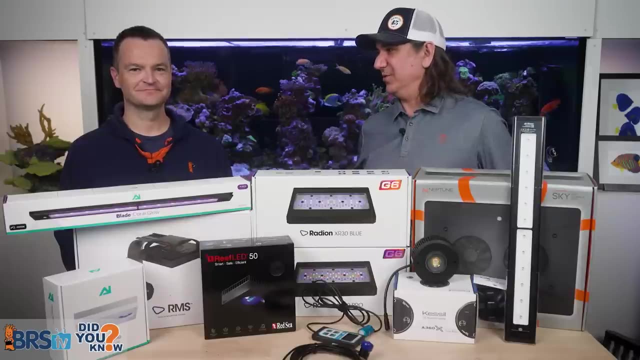 I would. I would tell you almost like probably like 92 out of 100 times, if I gave somebody an $800 light and a $200 par meter, Or I gave somebody a $1,500 light and I have no par meter and asked which one was more successful down the road. 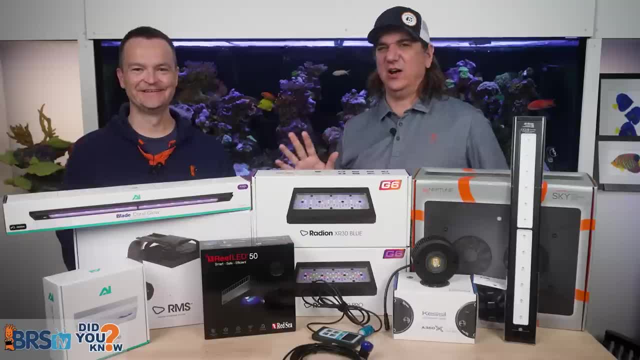 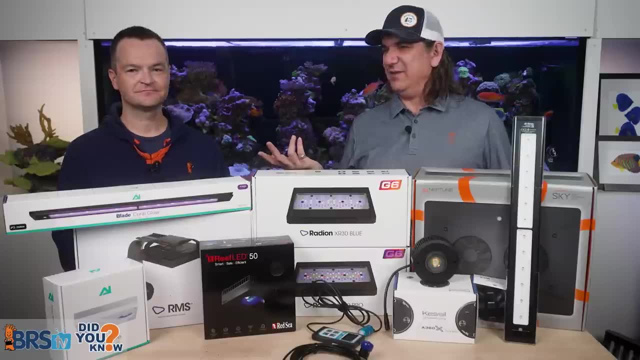 For sure, the $800 person with the par meter, like 93 out of 100 times would probably be true. And so, because we're tuning it to the organism and what it needs and what it thrives on, Now that par meter, though, again is that big one. 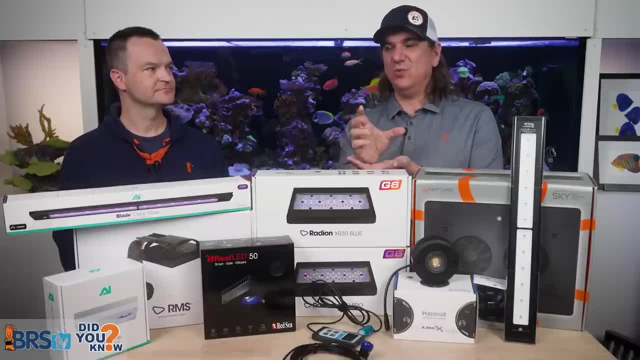 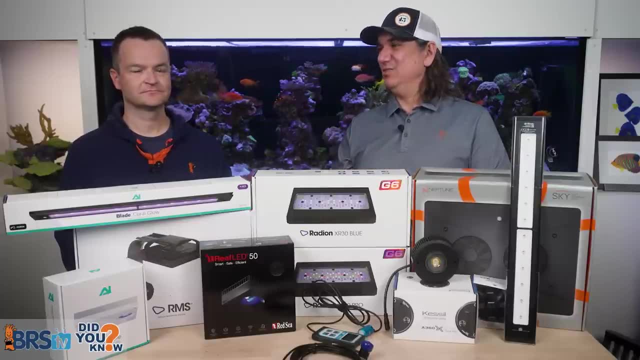 Like, just use it, like you can buy it, use it for up to two months, Let your buddy use it like loan it to your club, Do whatever you want to do, Do it with it. And then in two months you can actually return it within 60 days for just a small restocking fee. 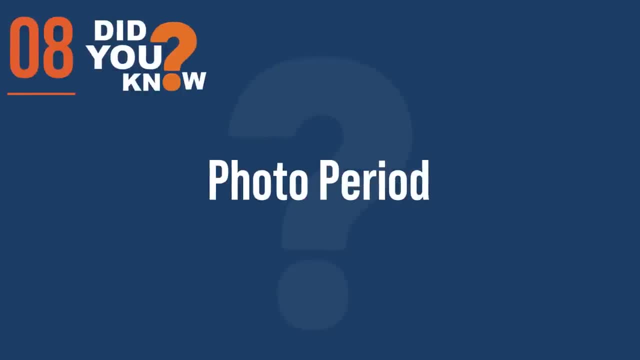 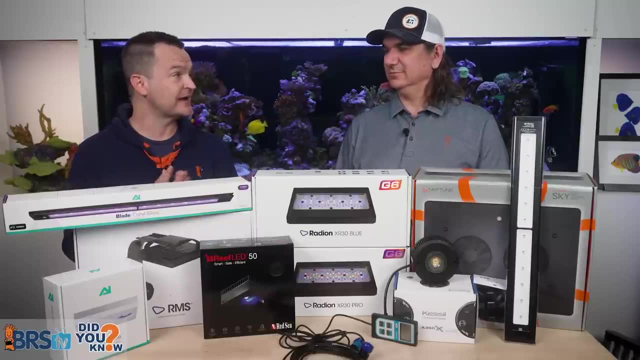 This is just a service, because we want to help you get it right. Number eight: we've got the spectrum down, We got the par down. But what about photo period? We found that about eight hours is the sweet spot. Now, if you want a little bit more time to look at your tank, then you can always extend that at the beginning or at the end. 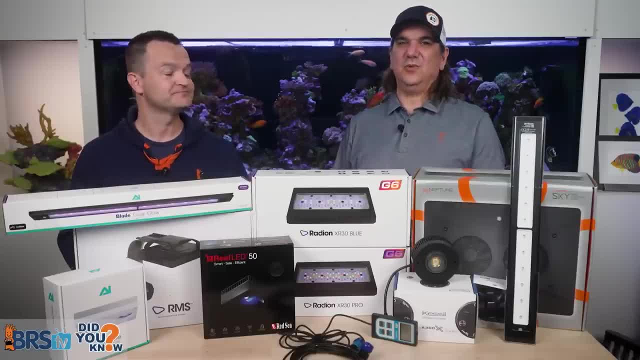 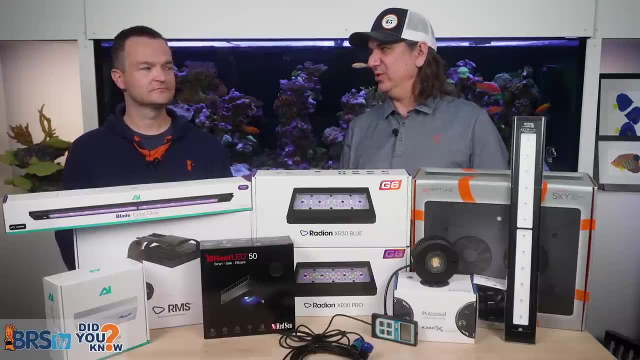 But make sure when you do that it's at a fraction of the par. The reality is, eight hours is just a Safe spot, right, Some people will go a little longer, Some people may even go a little shorter at peak, But the reality is is what you're doing is kind of like counting photons here. 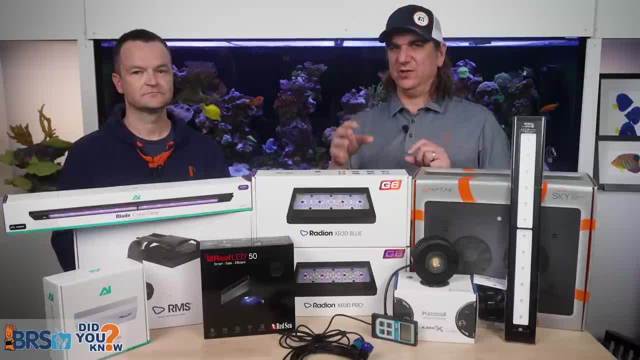 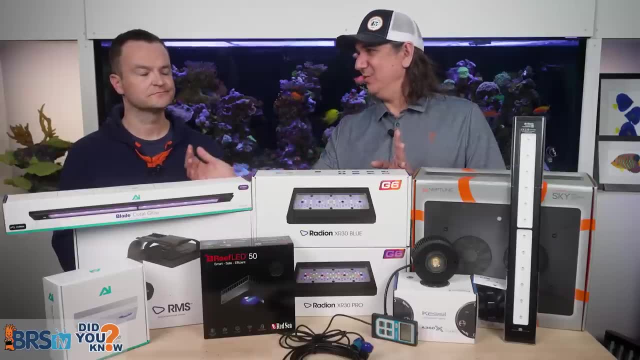 So you know, if I got 300 par, there's a certain amount of photons going there and it's eight hours. But if I had only 200 par I might actually be able to get the same amount of photons if it went 12 hours. 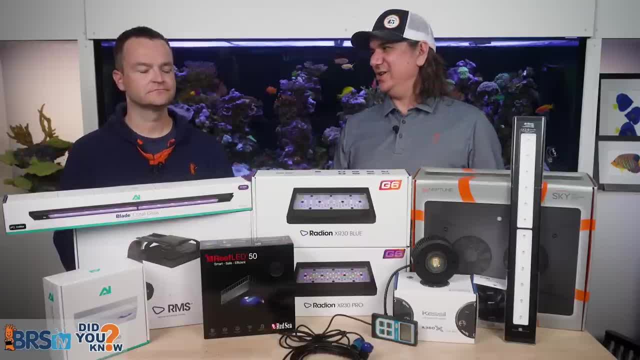 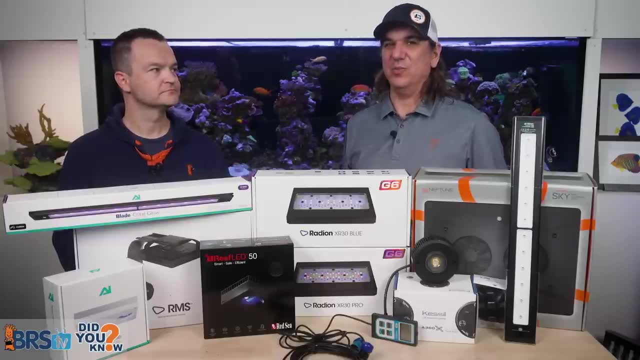 Right. The answer is like we don't know yet the equation there, but we do know that eight hours seems to be the area where a lot of people are really, really, really successful, or like almost everybody. That won't be the reason that you fail. 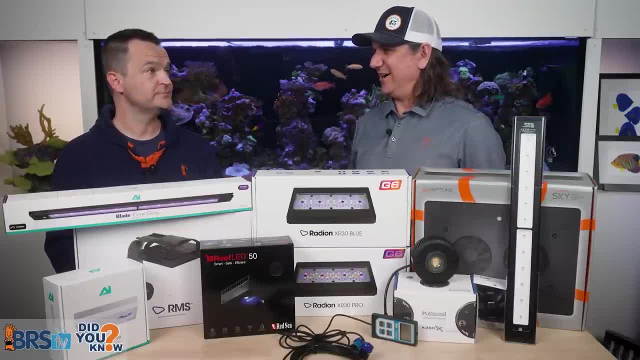 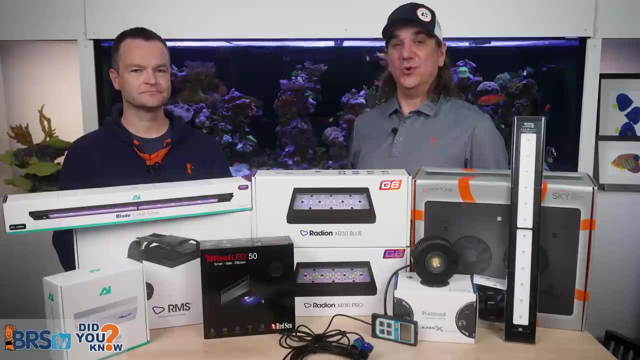 Now let's say you want to go beyond that. You want to just get into that DLI question which is like how intense and for how long? Alkalinity is your answer. So don't just like wing it and look at it, say I'm going to try nine hours tomorrow. 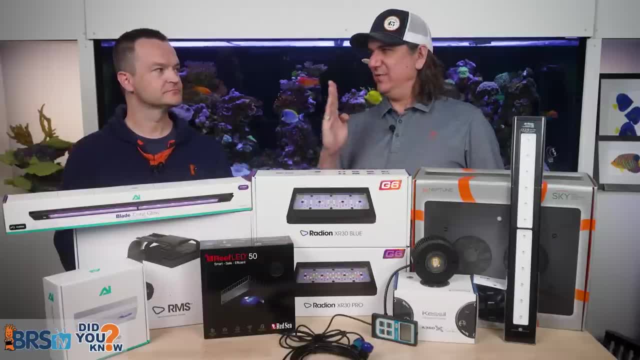 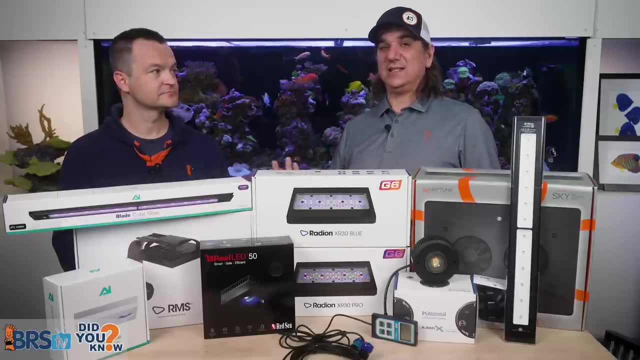 Do try nine hours, but like get a daily measurement of alkalinity every day, Right, And then tanks consume in about this much every day, And then I crank up the lights and if I'm doing something good for the tank, like extending it another hour, 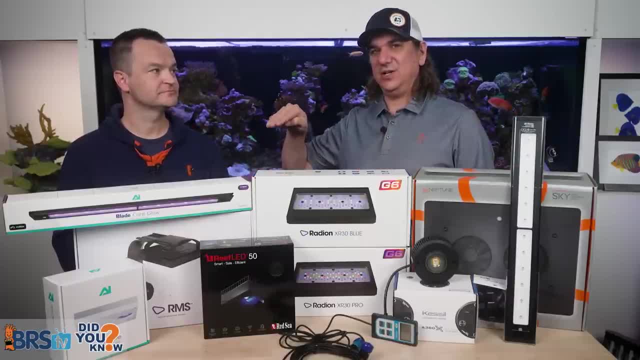 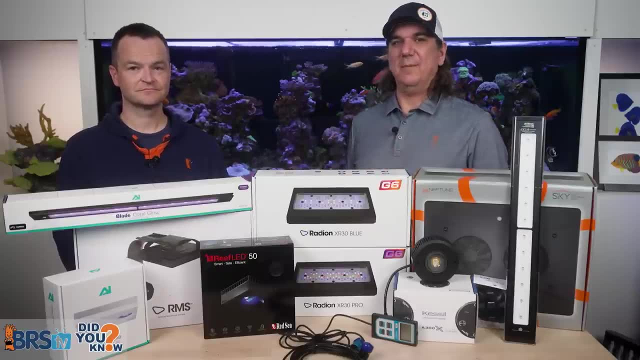 Well, in that case, I should probably see the alkalinity drop. because it's consuming more. It's telling me: hey, yeah, I appreciate that extra energy, I'm going to reward you with more growth. But if it actually does the opposite, 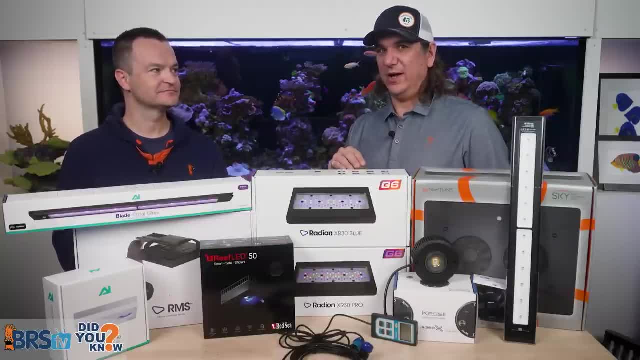 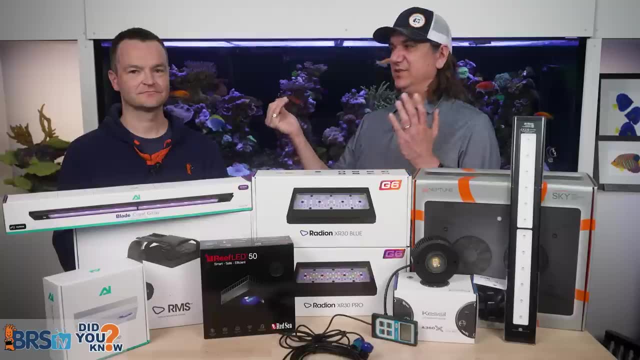 like, say, I crank my lights up 20% and go from, like you know, 275 par and I really want to push the limits and going above 350 or something. Well, if all of a sudden the levels in your tank go up, 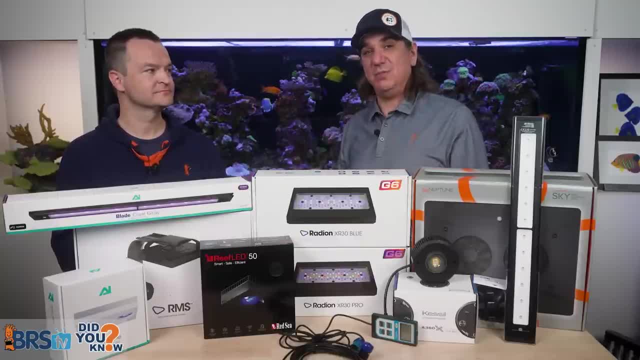 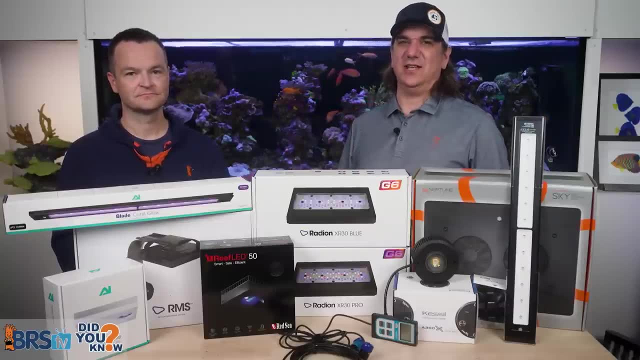 it means the corals aren't sucking it up as fast as they used to, which means you're hurting biology. So that's the nerdy end of the photo period, If you just want to know that you did it right. eight hours is that safe sweet spot. 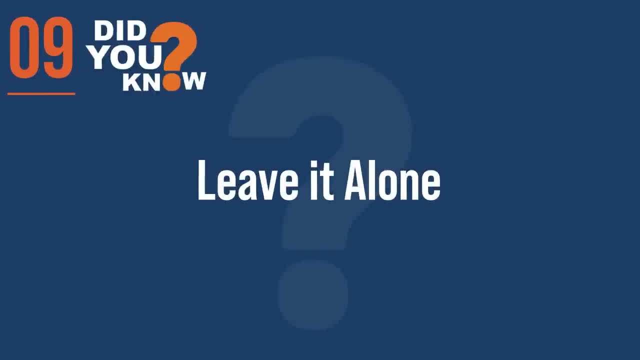 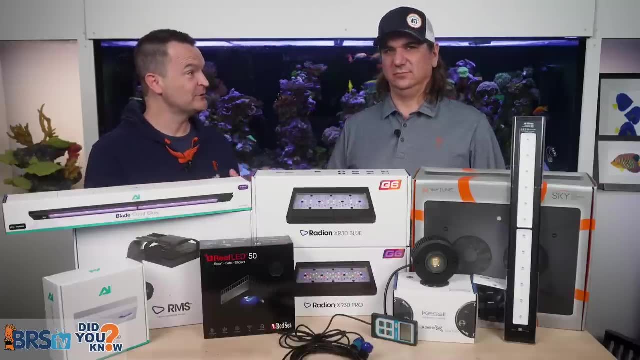 Number nine: leave it alone. I'm going to say it again: Leave it alone. Somebody who toys with it, who tinkers with it, is probably what 10,, 20 times more likely to do harm to the corals than to actually help them. 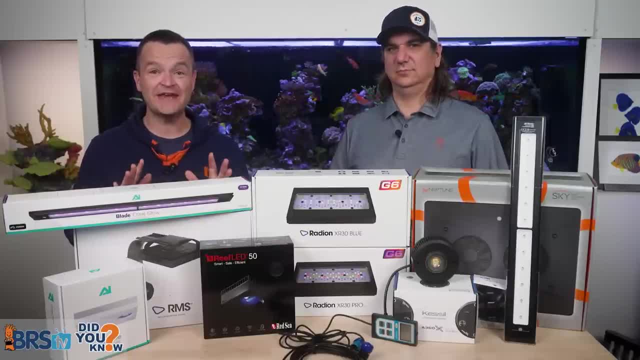 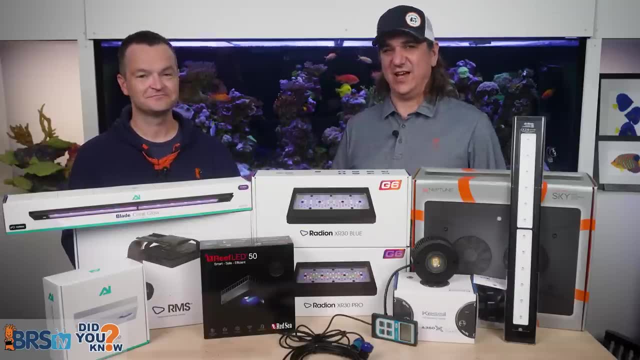 I mean, I mean it. I mean it. Leave it alone, Don't mess with it anymore. It's really not a toy. that is not a toy. lighting Junkies just have a fraction of the success of those that do it Well the first time and then have the confidence that they did it. 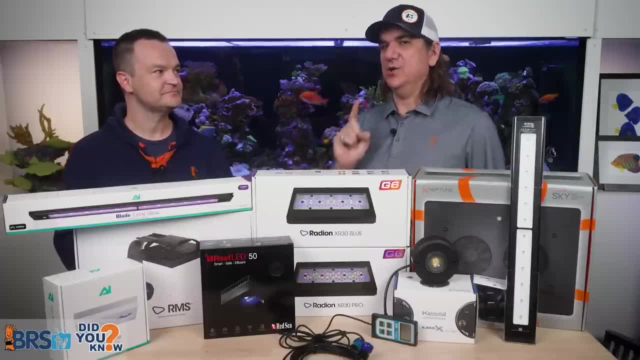 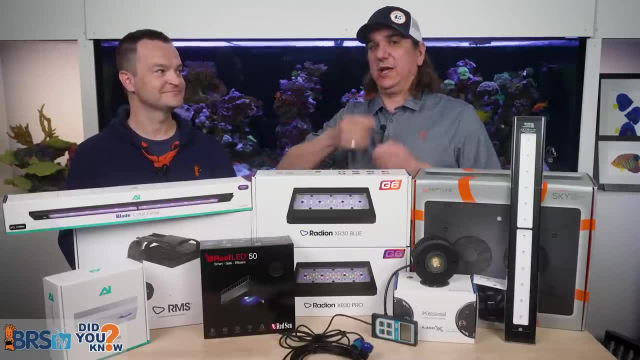 Well, regardless of, like some bumps they might see, they'll know: No, I got this lighting thing cover, I did it right and then leave it alone. Those people will be so much more successful than the people are like trying to constantly adjust things to fix something. 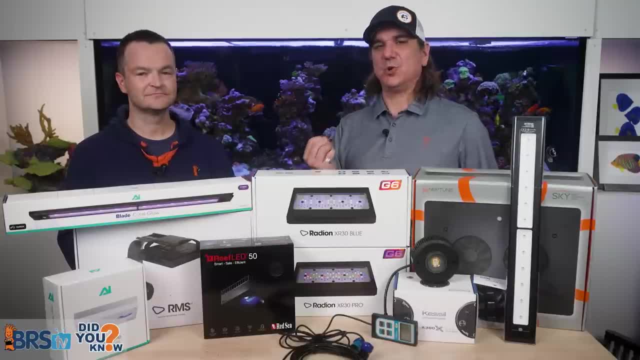 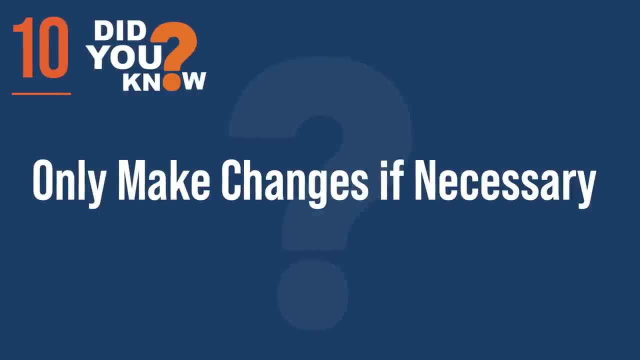 They didn't know. so find the confidence, Understand what you're trying to achieve, Do it to the best of your ability and leave it alone. That is where the best tanks come from. Number 10. Let's say you set it up. 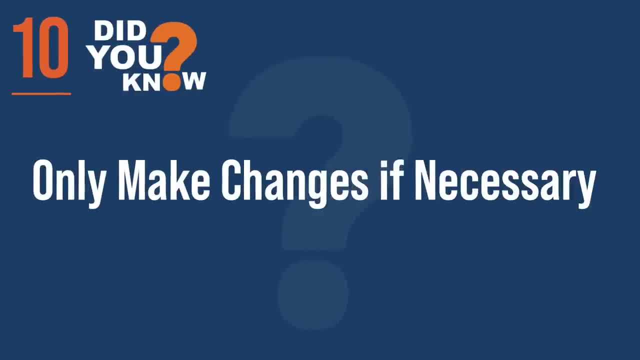 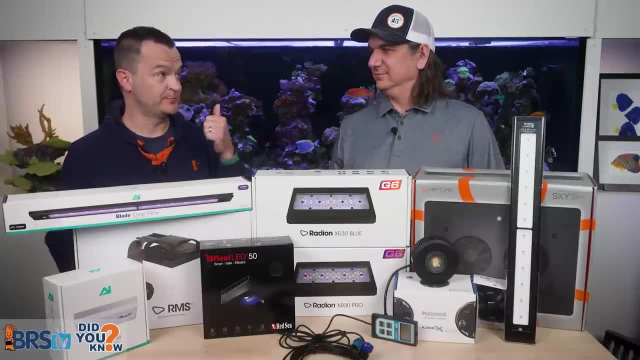 You did it wrong because he didn't watch any of our videos. You can make a change, but only do it when you know you've made a mistake. But when you make that change you need to make sure you plan it out really well. 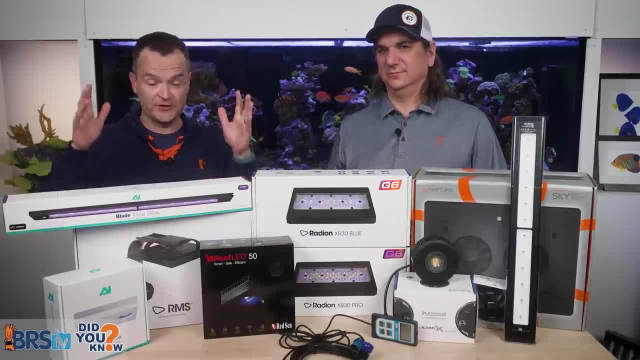 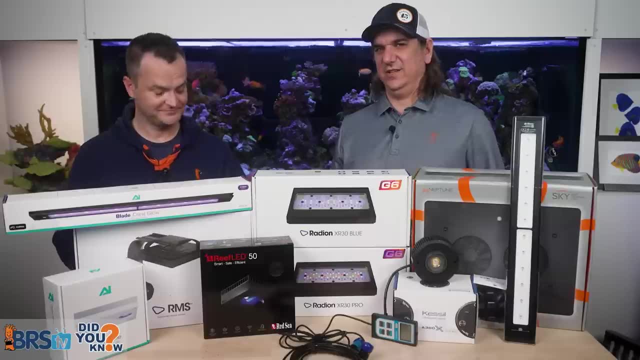 The change needs to happen slowly and your change needs to be good for at least two years. You need to make a change that's going to be permanent and you're not going to touch it again. I would go even further than this. I'd say, like, unless the tank is actually suffering in some way. 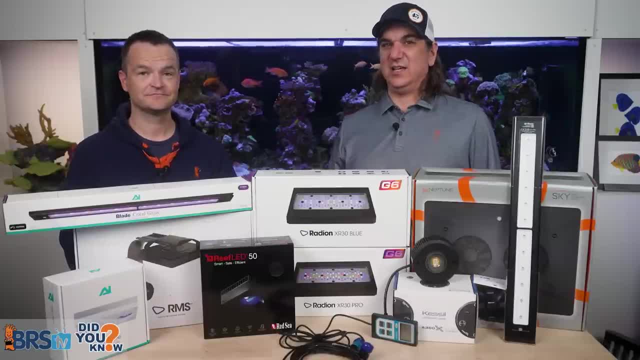 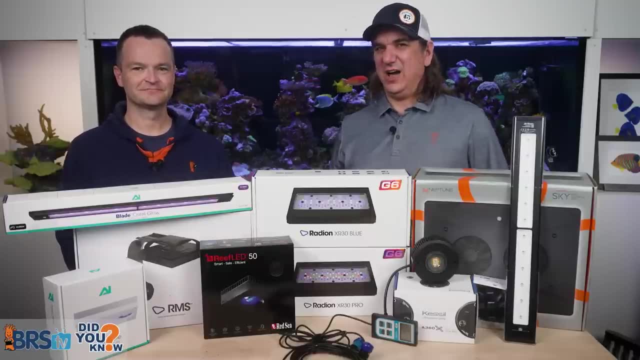 Clearly, the biology is not being served like, because if everything's going well, sometimes you can do less than perfect and it will still go well. Okay, but like now that you know what you need to know. if you're like you know what man, this is going to go south for me. 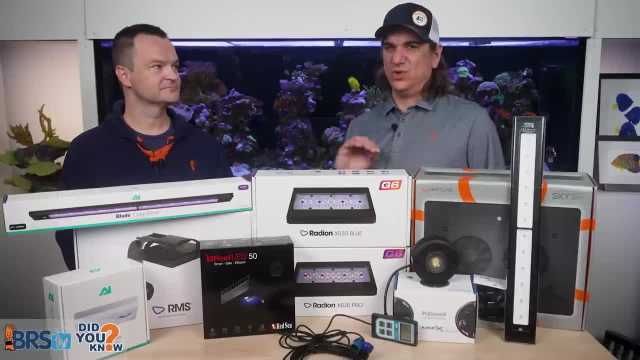 I don't actually have to wait for it to go south, So like, for instance, this is really common with SPS owners. It's like I put in these Little modules everywhere and I don't know there seem to be doing really fine. 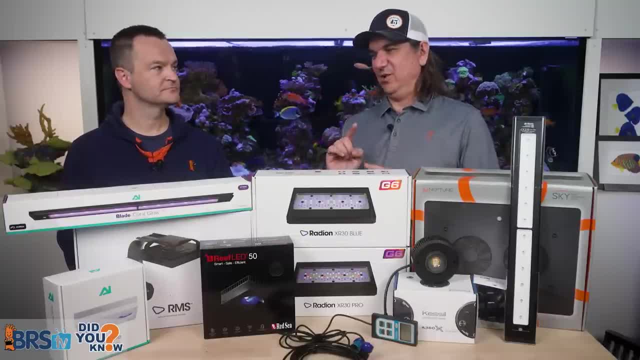 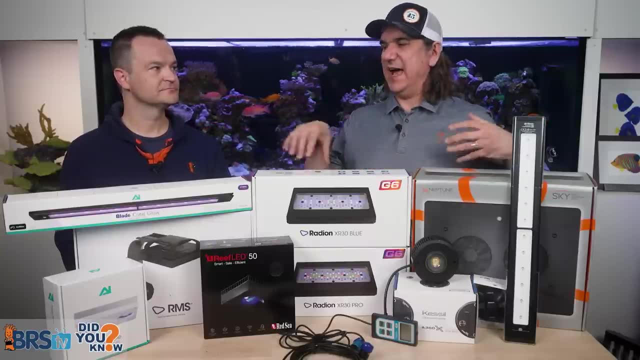 My little frags are growing. It is absolutely true that growing this little teeny frag is totally different than growing a colony that shades itself and its neighbors, And at some point you're going to have to add in the fill light. So well, you know what, though?